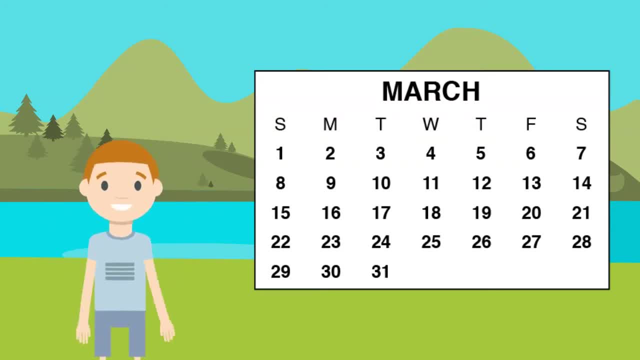 Let's go over the days of the week. The first S is Sunday. Sunday is always the first day of the week. After Sunday is Monday, then Tuesday, Wednesday, Thursday, Friday and finally Saturday. Saturday is always the last day of the week After Saturday. a new week begins with Sunday. 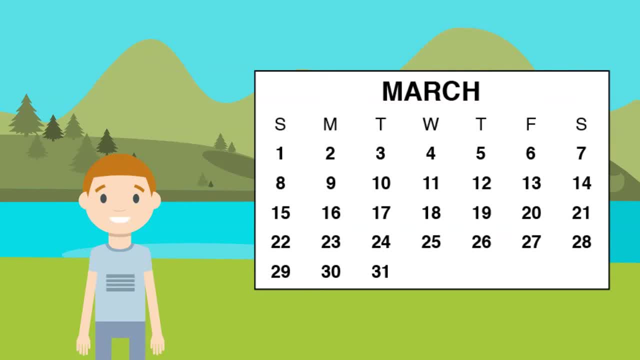 Did you notice how many days are in a week? Yes, That's right. There are always seven days in a week. In this month of March, there are four full weeks, with three days left over. What is the last day of the month of March? 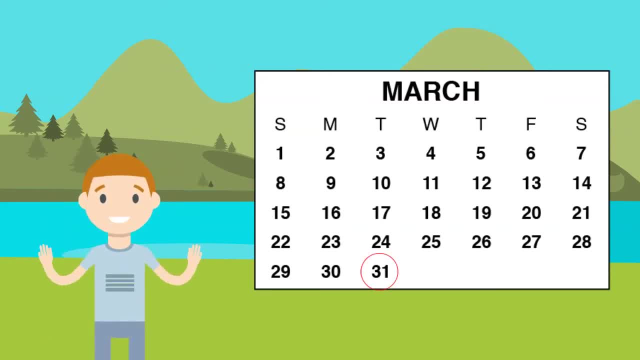 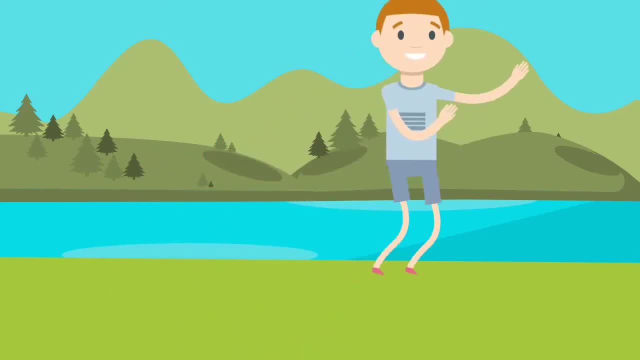 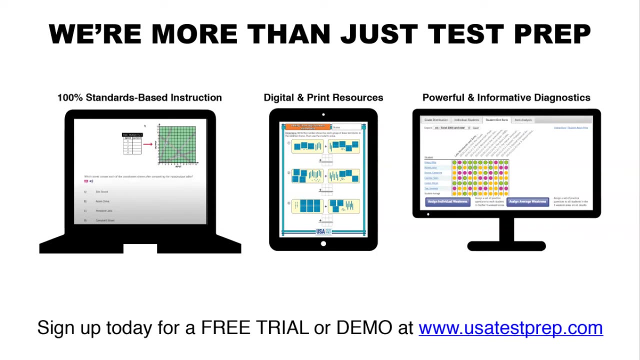 Yes, The 31st is the last day of March. The day after the 31st starts a brand new month. Follow me to learn more about the month of April. Your video will continue in a few seconds. For more videos like this, along with great standards-based instructional courses and powerful diagnostics, visit usatestprepcom to sign up for a free trial or demo. 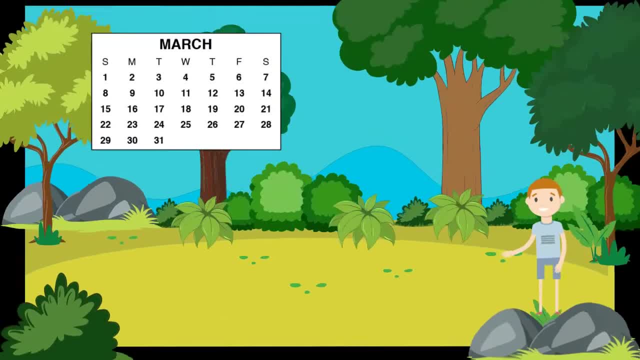 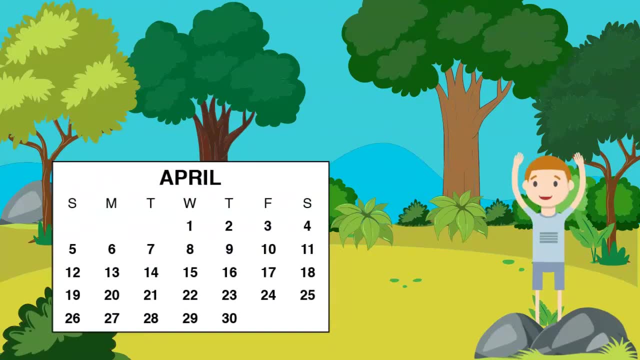 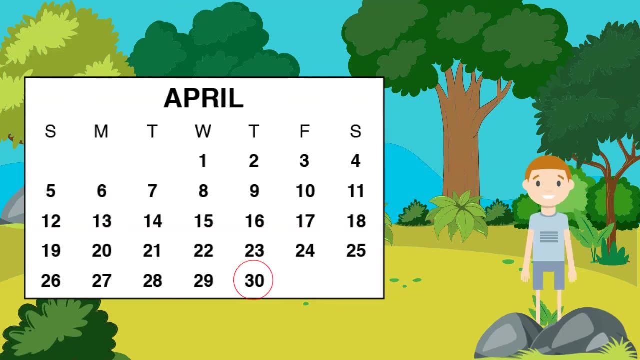 Your video will now continue. The month after March is April. The day after March 31st is April 1st. We are now in a brand new month. How many days are in the month of April? Great, There are 30 days in April. Most months have either 30 or 31 days. 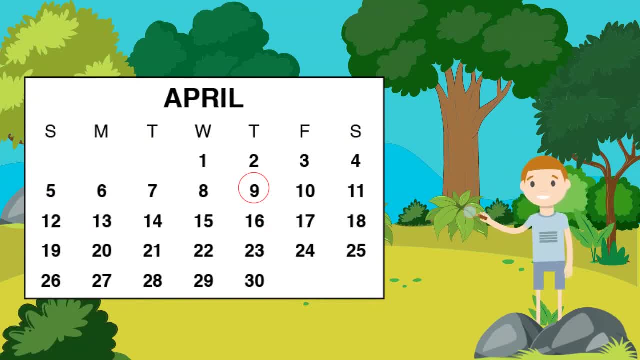 Find April the 9th on the calendar. What day of the week is April 9th? Awesome, April 9th is on a Thursday. We look up above the 9 on the calendar to find the day of the week. What day comes after April 9th? 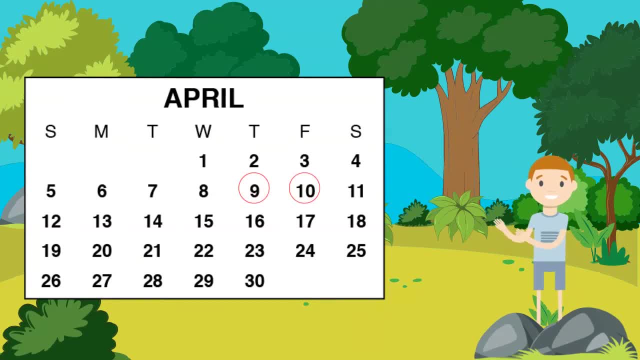 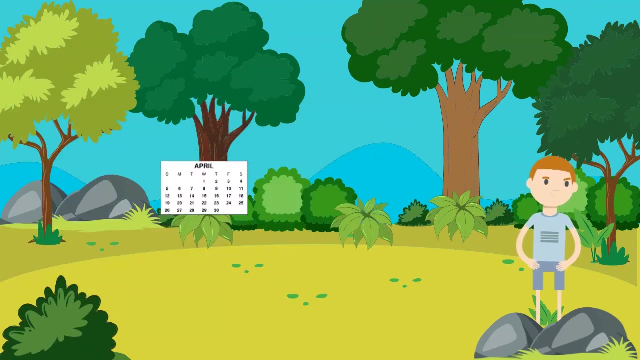 Yes, April 10th comes after April 9th. April 10th is the next day on the calendar. What day is exactly one week after April 9th? April 16th is one week after April 9th. To find the next week, you just move down to the very next row.